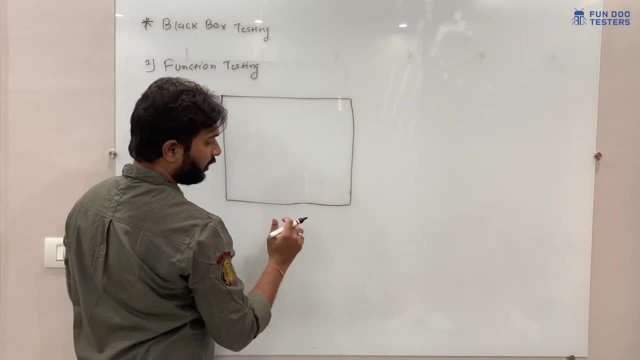 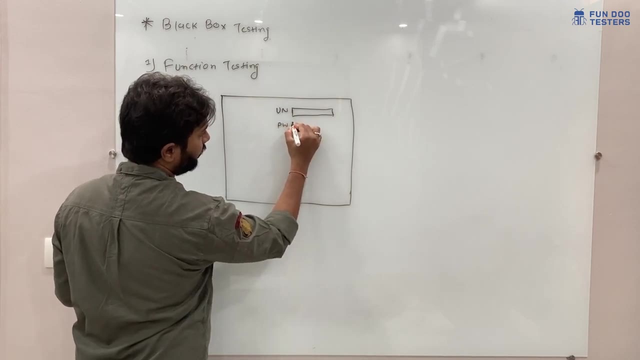 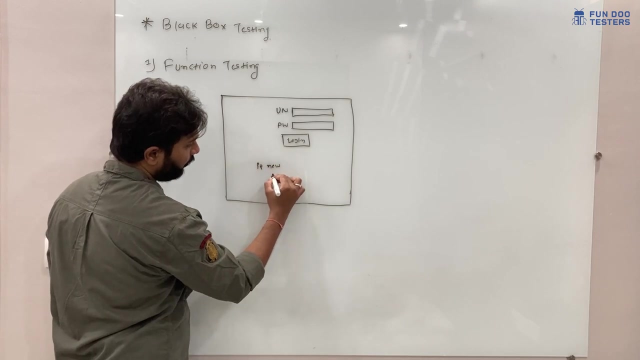 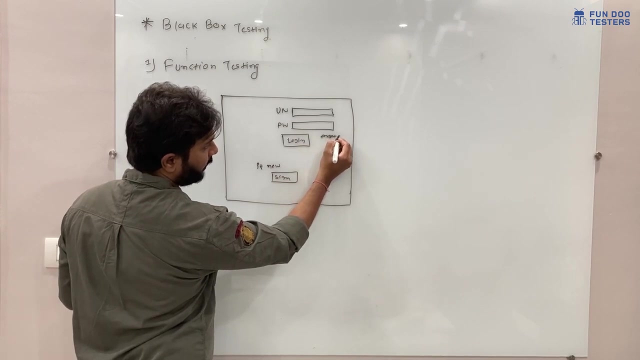 web application. so this is how it is it looks. we have username field. later on we have password field. we have login button. later on we have if some website has got written, if you are a new user, then you have here sign up button and here forgot password. forgot password if you are going to. 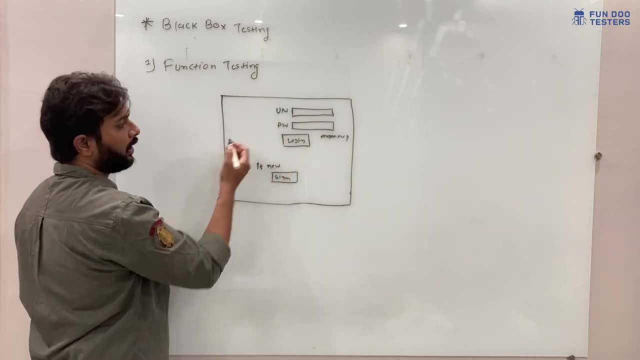 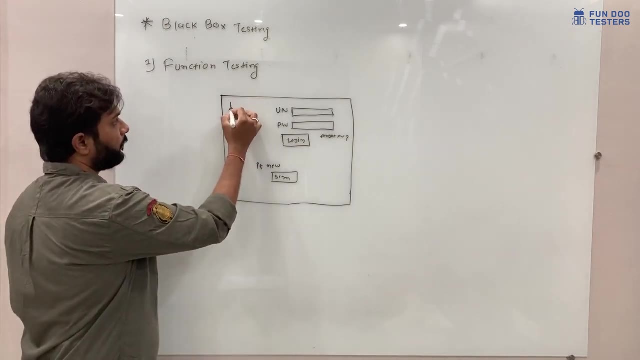 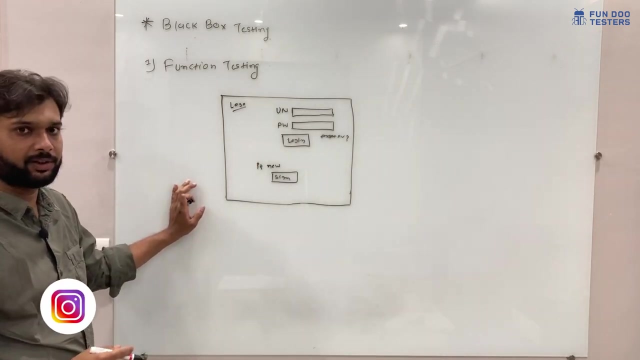 forgot the password, then you can click here and you can recover your password. apart from, this page has which data? so this page can have company logo and few advertisement or few other buttons. so now we are going to perform the functional testing. so functional means, as per the definition, 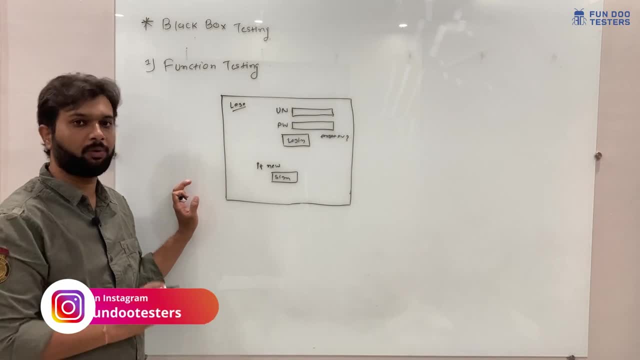 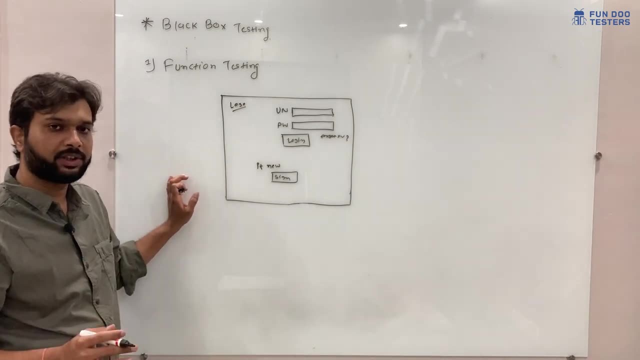 we have to test each and every component thoroughly against the requirement specification. so now question comes: what is the requirement specification? in earlier, in software engineering model or htlc models, we understood what is the requirement phase. so in requirement phase client has given all the requirements or in crs or srs documentation. if we are going to check they are. 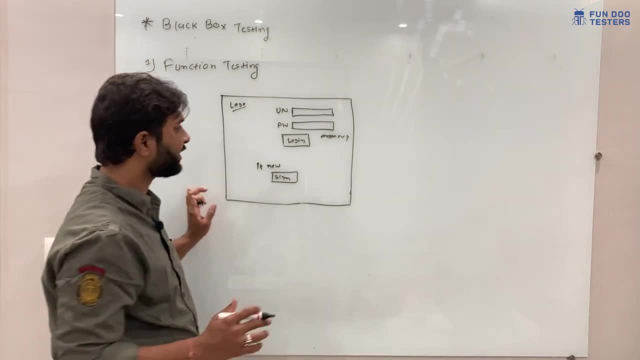 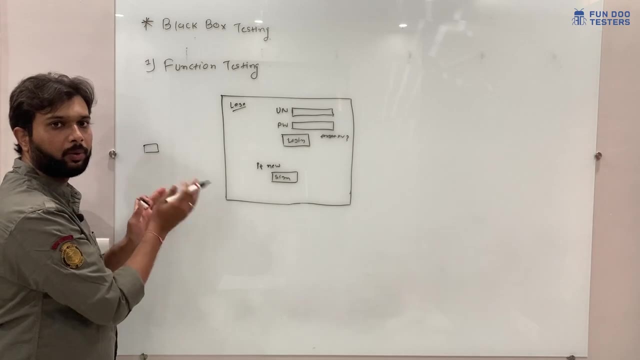 going to mention each and everything in detail. so, for example, let's consider for the login page, so login page, what they have mentioned, which are the algorithms they are going to use, but it is going to a part of the white box testing. but still, we are discussing here the only 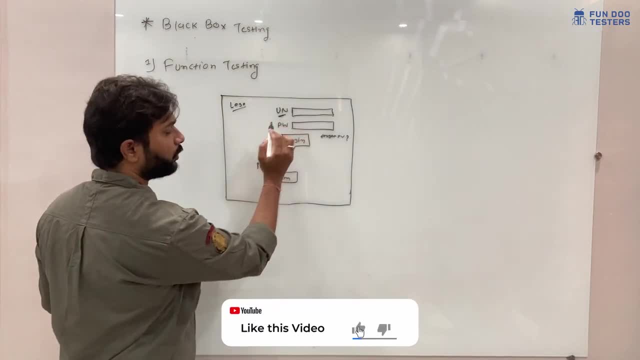 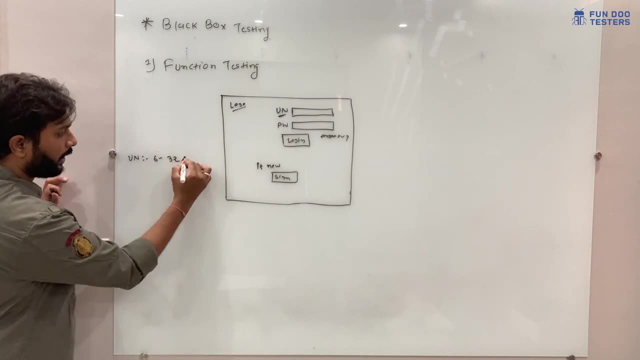 first start testing. so for username field there are certain requirements. so for username field, for example, in username field is going to accept 3 to 32 characters. later on it can have a numeric and alpha numeric. so this is my first requirement. second requirement: numeric and alpha numeric. 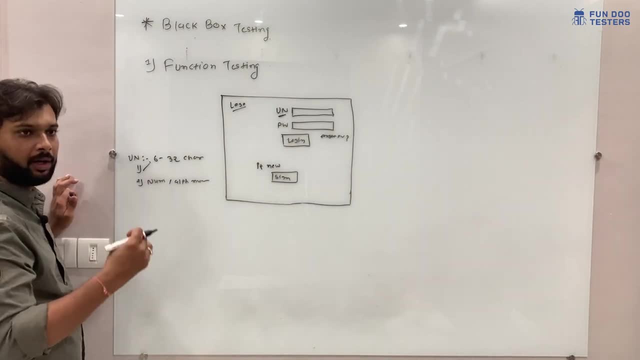 after that it has to be unique. so, for example, if i am logging to any application using my gmail gmail id, contacting correct from to testercom, so no one can use that gmail id or that mail id. so it has unique email or unique username- unique username. later on you cannot enter the special character or emojis if you are going to open the any. 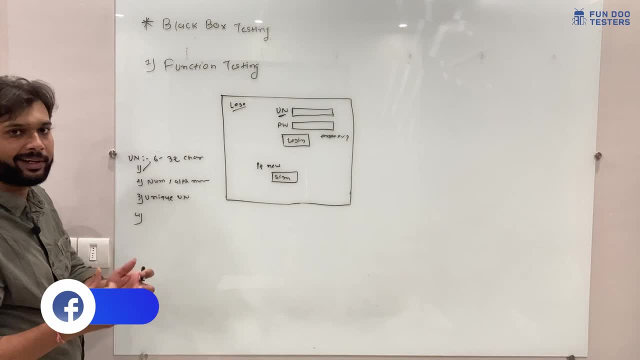 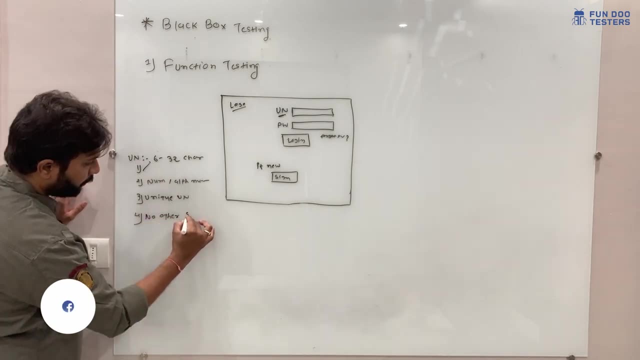 mobile field or anything you can have in keypad. you can enter anything, but this field is restricted with the, these two characters, so no other special characters. later on we are going to look for the password. so password also. we have the same requirement. password also. first level 6 to 32 b. 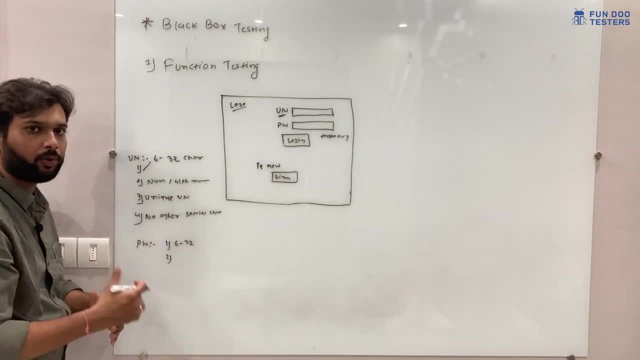 then in password there are few extra conditions to enter special ones. so passwordy features. IMOJI腼 Croixo ain, most passwordy features. what to add? interested м Are to add special or based on the application they are going to add the extra validation. for example, if you are: 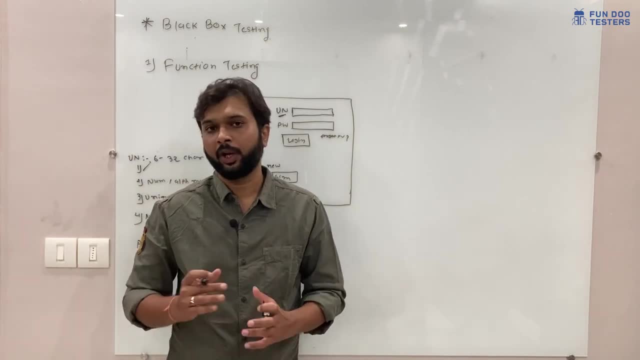 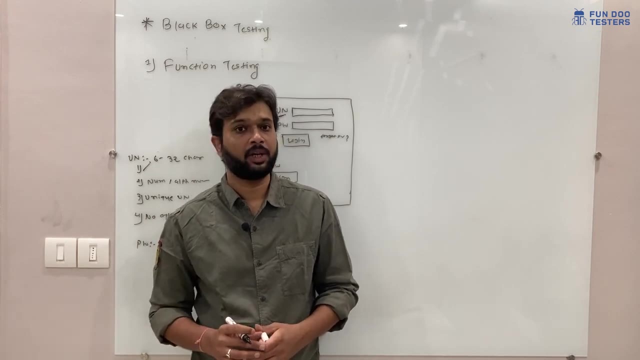 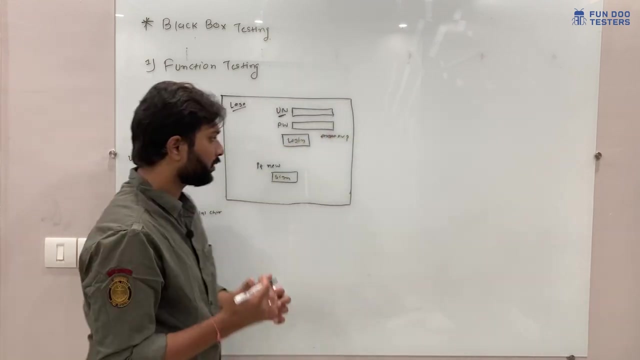 talking about the simple application or normal blog post or anything, you can have any password. but if you look about the other applications, for example more secure applications like bank applications or schooling software or health software, so it can have little complexity how it works. so generally, what happened in the password field? they have given some requirements. 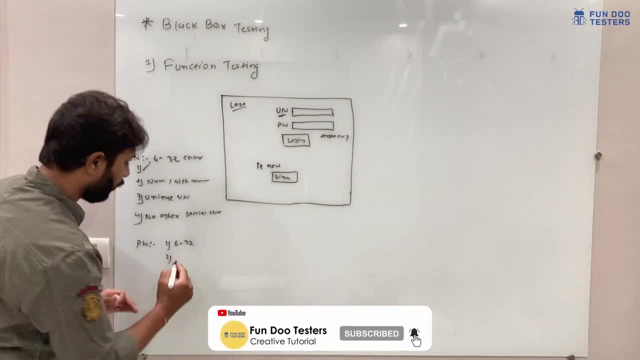 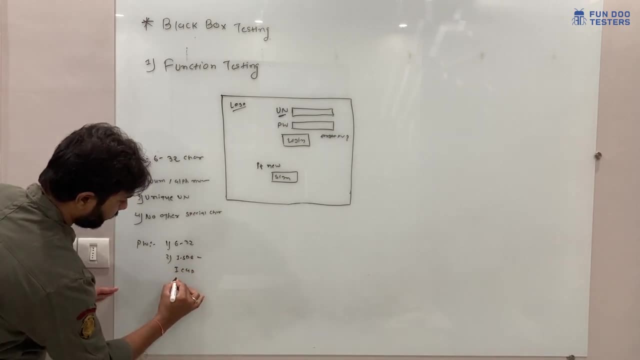 so it should be 32 bit. then it should have password, should have one special character, one capital letter and small letter, for example, four small letter and total length will be 6 to 32. so it has to fulfill this, all the criteria. so this is how password field work. 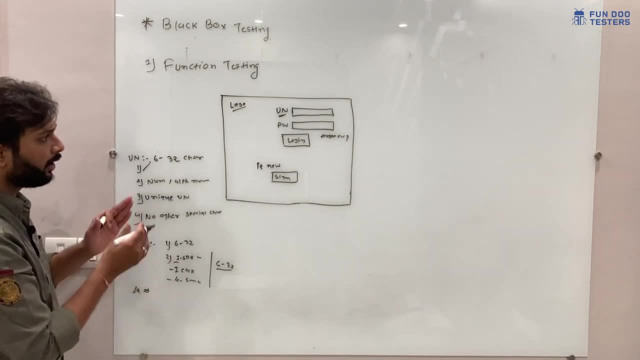 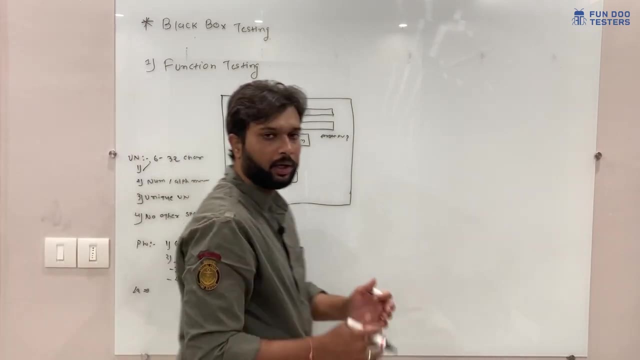 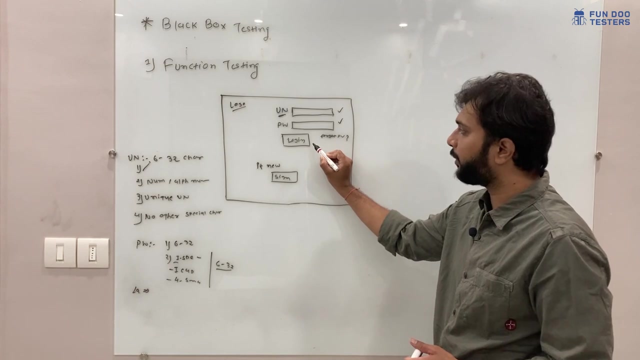 and there will be a login button. so in login button we only check if, after entering the username and password, login button is the functional or not. so what happen in the few applications if you are going to? if you are entering username and password, after that only login button will be enabled. enable means before entering it will be light color. 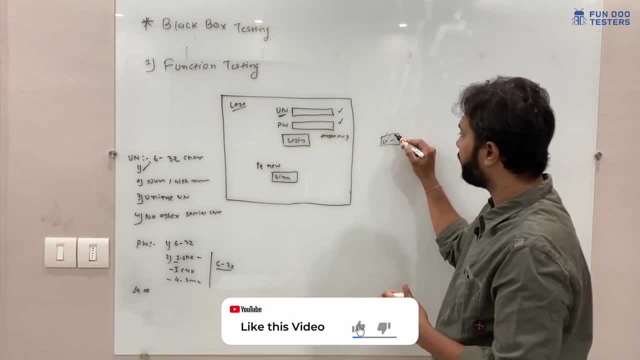 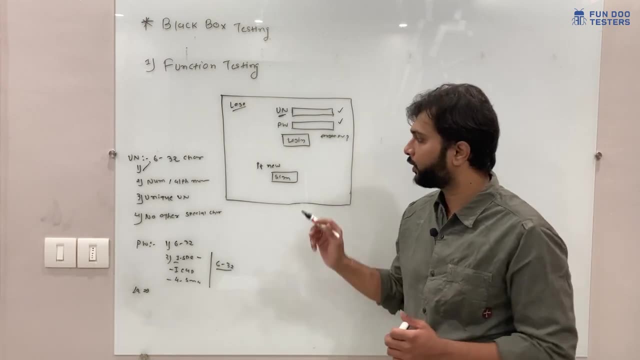 so once you enter the data, it will be pop-up or it will be highlighted or it will be dark color. so this is called once you enter this data. after that, only this will get highlighted. so this is the another requirement. later on it can have multiple other requirements. so what other? 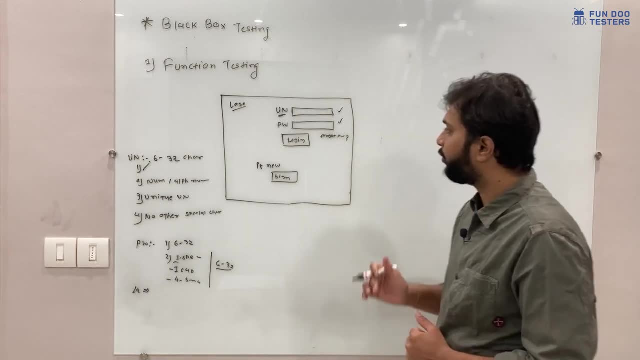 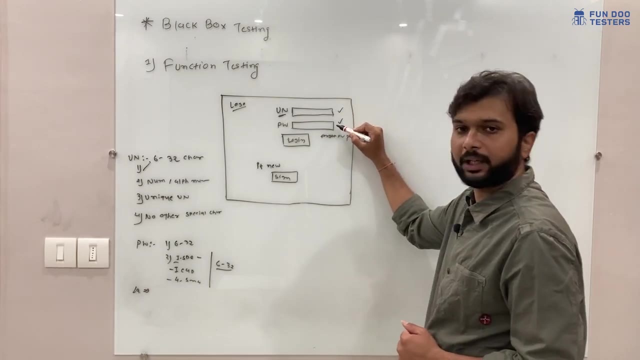 requirements can be, or have you ever observed the login page so it can? for example, let's say, if you are missing this field, username and you directly, you are done, you are going to directly enter the password. so by the time login button should not enable otherwise, what? 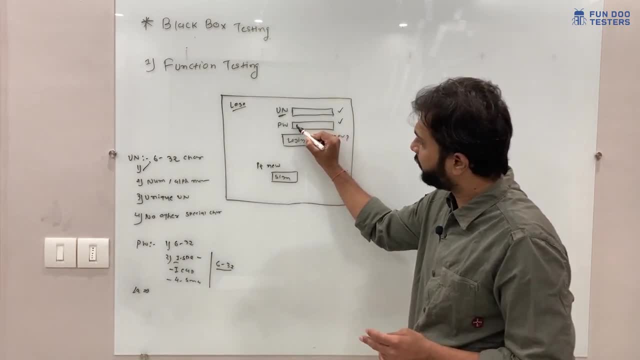 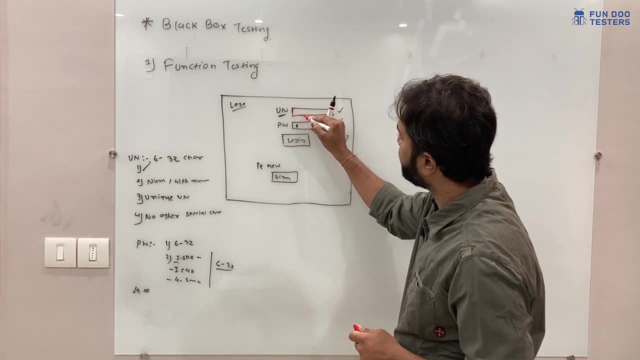 happen in few applications if you are directly clicking on the password button so you can see mouse over here. so by the time this field will display the error message, or this field will become the red instead of black, it will become red and here you can see the error message. and here: 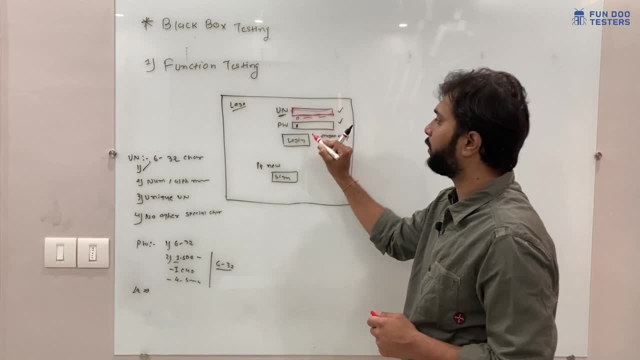 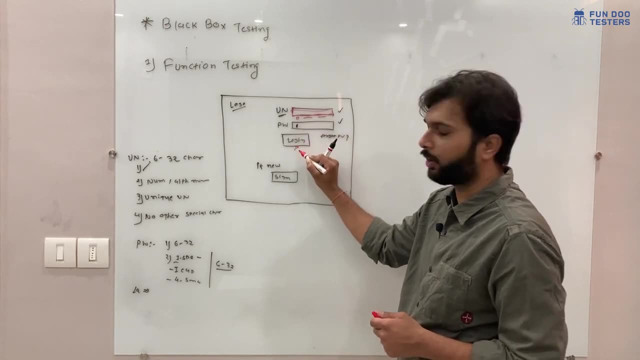 it will display the error message. please enter valid username. or sometimes it will. if you enter the username and you are not going to enter the password directly, you are going to click on the login button so it will display. this field will get red, or error message will be displayed, or 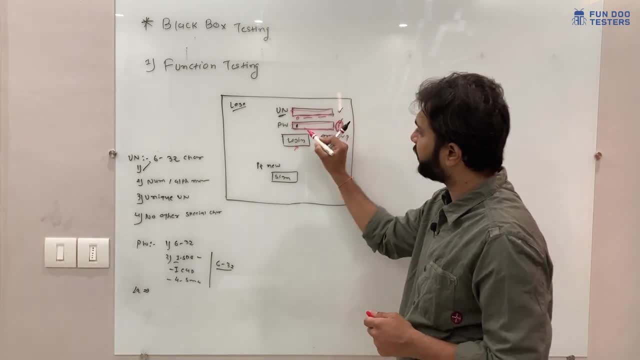 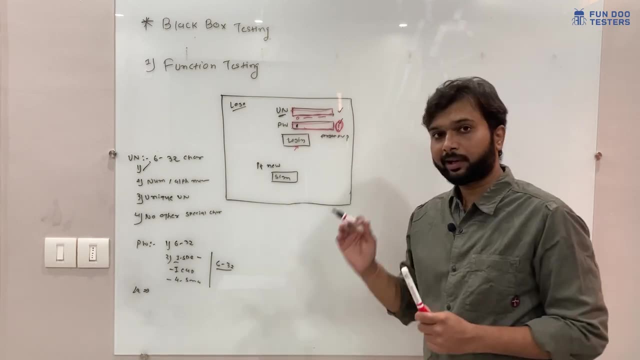 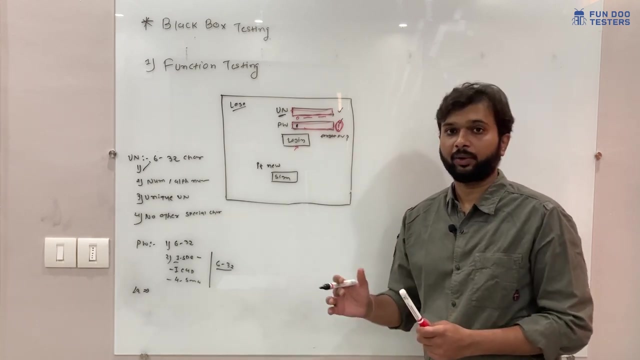 some time. experimentary sign will here. it will be pop-up and equal, as please enter valid password. so this is the basic validations and this validations are called as a client side validation means we are logging through the any browser or any android application or ios application, so 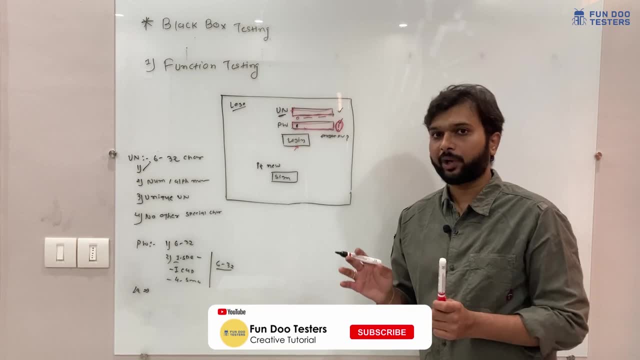 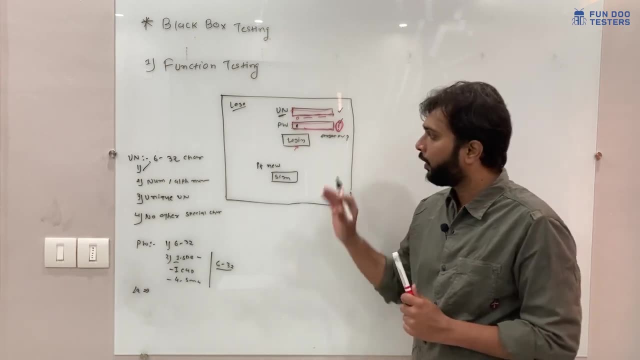 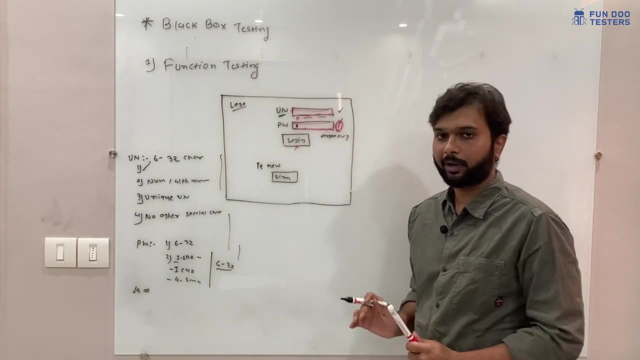 this. applications will work as a client, so don't worry about this term. we are going to discuss what is a client and what is a server in depth in further session. this is how application will work and this will be. this is the how requirement looks, so now we need to test this requirement. 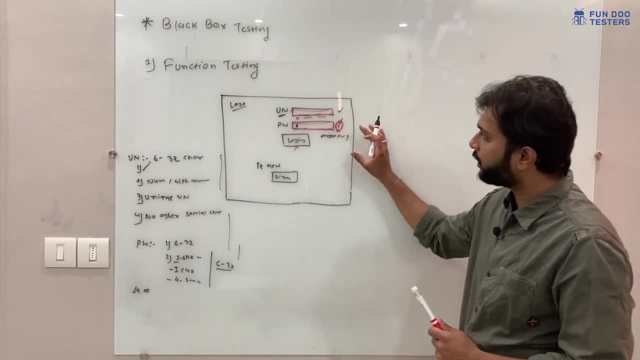 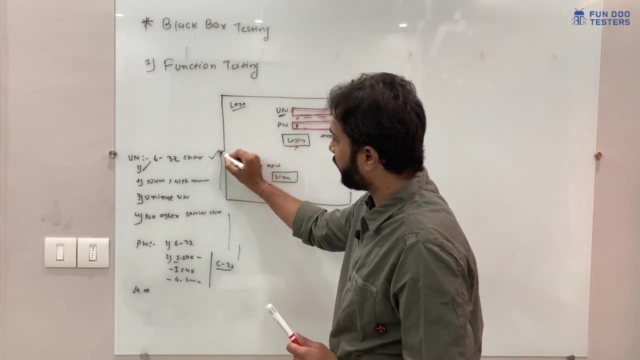 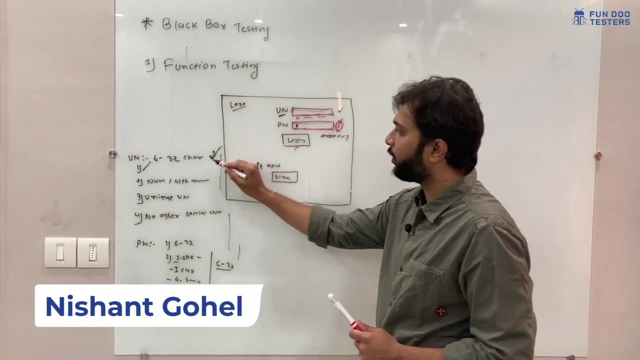 thoroughly. so how can we test this requirement? so, based on the scenario, we have to write a test cases. so first, what we are going to do, first we are going to check this requirement. this is my first agent. i am going to test only this requirement. so what happens, first i am going 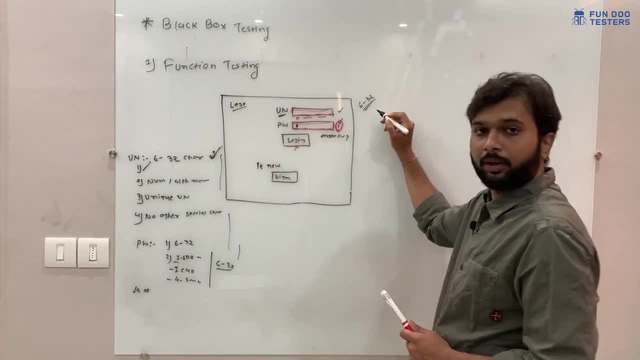 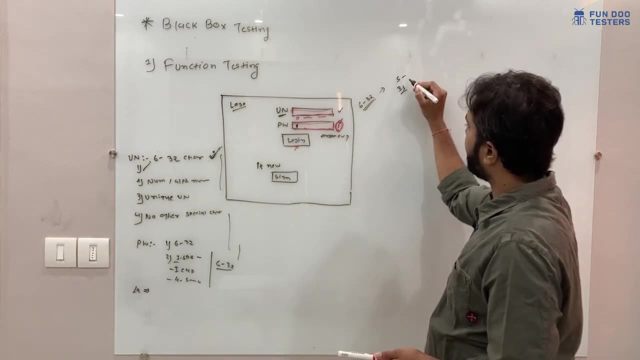 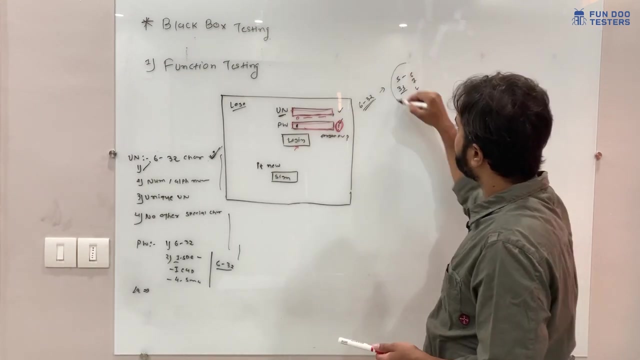 to enter 6, 6 to 32 character. so i will add 6 to 30 character. after that i will try 5 character, i will try 33 character, i will try 6, 7, 8, 9. so there are multiple ways i can enter. so this is again. 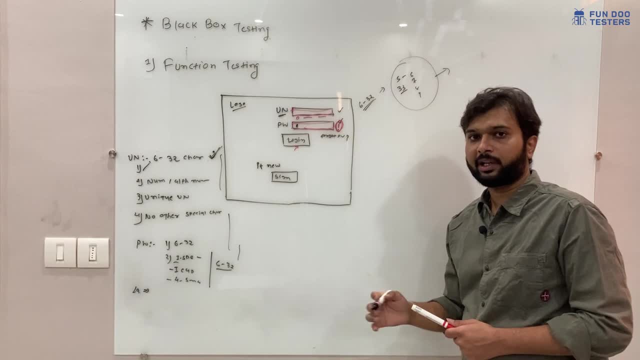 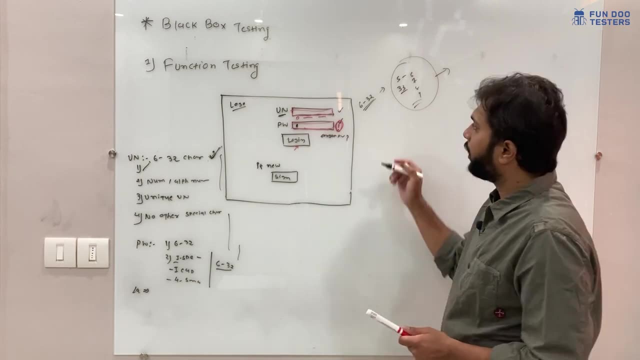 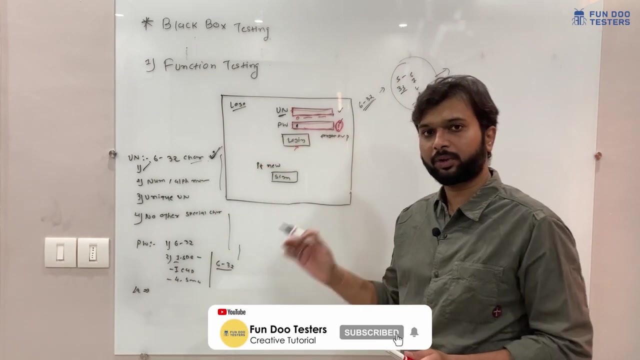 it will be a test design technique. so boundary value analysis, error guessing analysis, so this is called test design technique. so this also again we are going to discuss in the in test. but first question is: what we can test is 6 to 32 characters. if it is accepting 6 to 32 character, 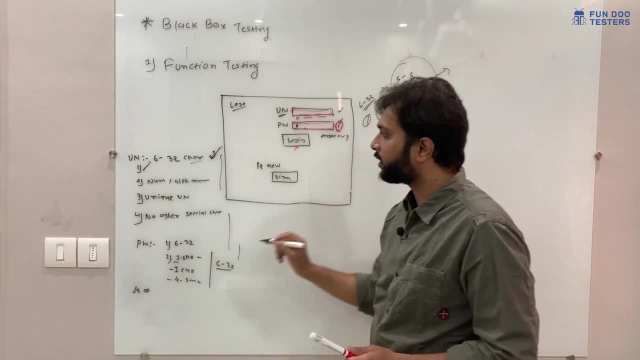 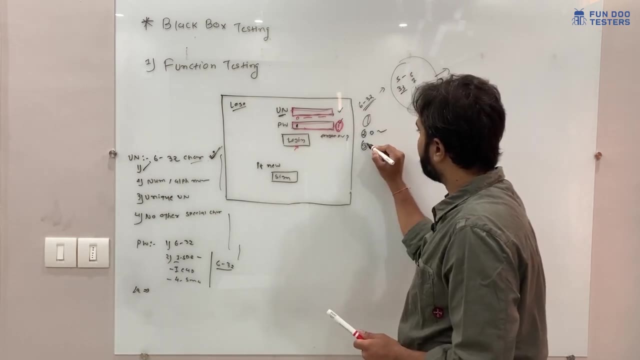 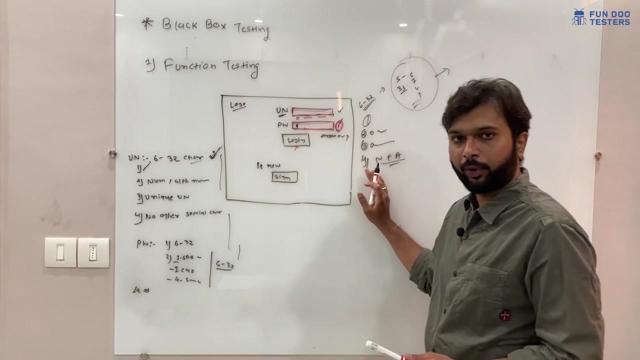 or not. so this is my first test case. another test case will be numeric or alphanumeric. it should take numeric alphanumeric. second will be only numeric. third will be only alphanumeric: alphanumeric, then numeric alphabets. with these two requirements, i can have four test cases. later on we can have a unique test, unique username. so, for example, i am going to enter: 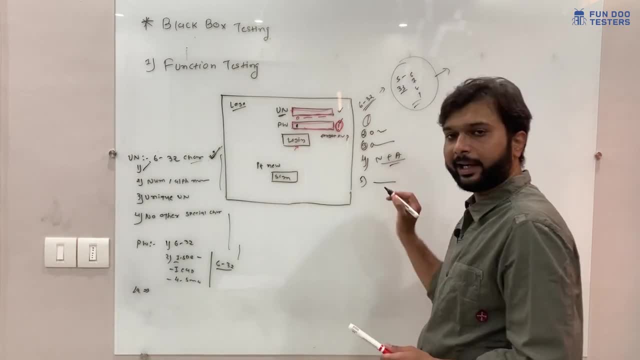 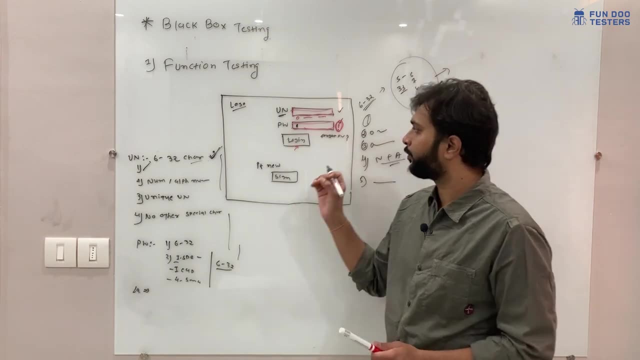 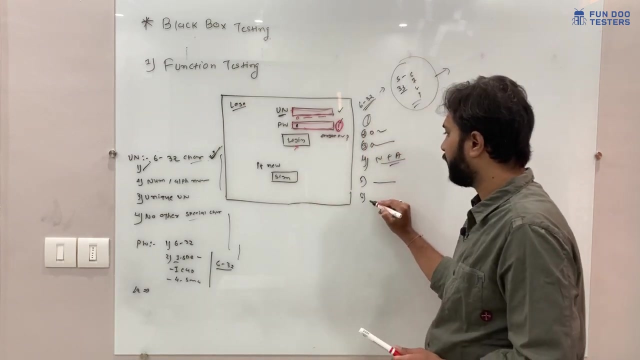 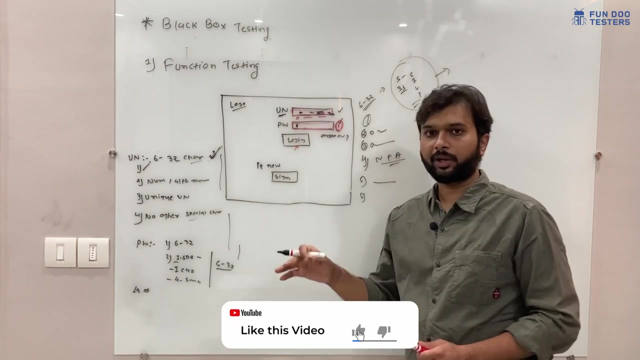 fundutester at the right gmailcom. so this has to be my username. it has to be unique. if it is not unique, then error message should be displayed. so this is my fifth test case and then no other special characters. so, for example, sometimes what happens? application is not itself allowing to enter me at the red star or minus or plus. it is not allowing. 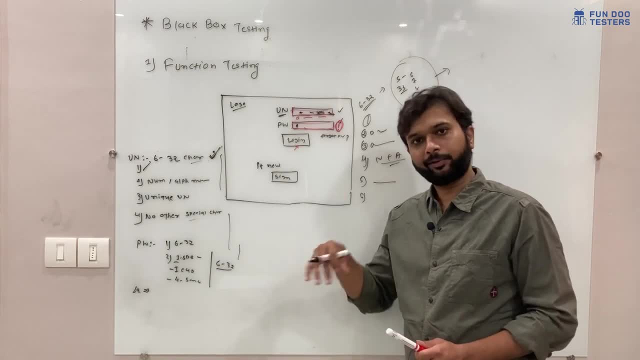 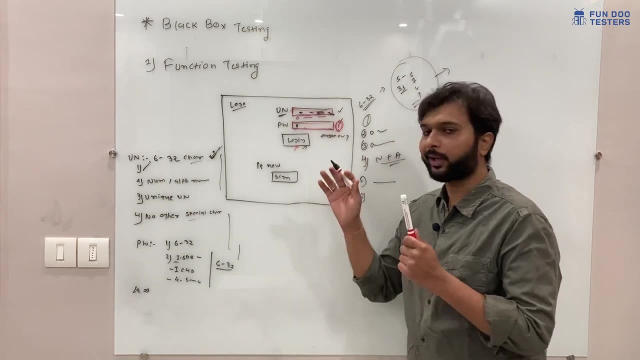 me to enter, but sometimes what happens? it will allow me to, it will allow me to enter, but while logging it will display the error message. so these are two different kind of variations. so what it has mentioned in the application, based on that, we have to verify. so we have to verify. 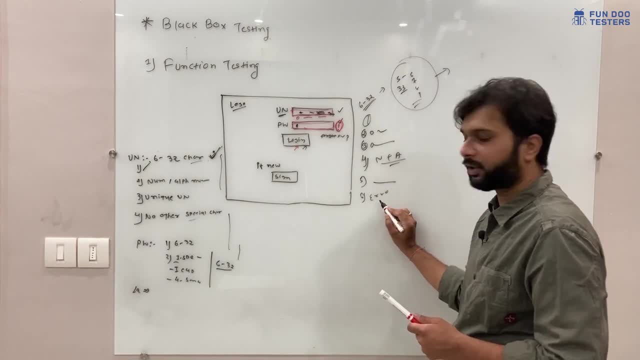 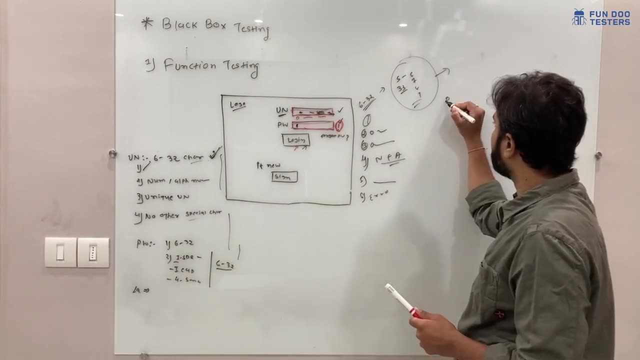 the error message. so this is my sixth test case of the username. similar way, i can have four passwords to password what i can do. for example, i am going to test the password. so my first scenario will be 6 to 32. so simply, i have to test 6 to 32 with this scenario. second number is: 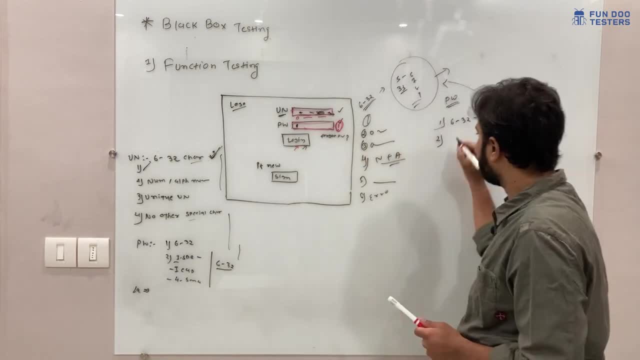 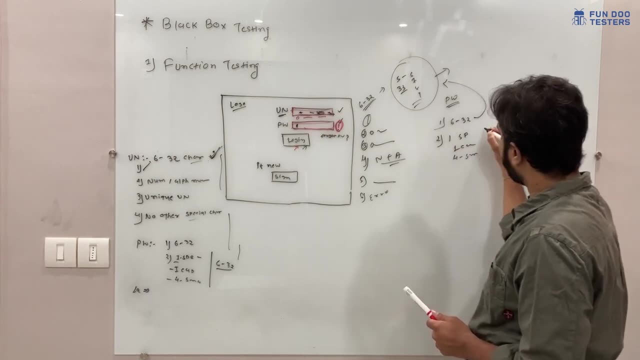 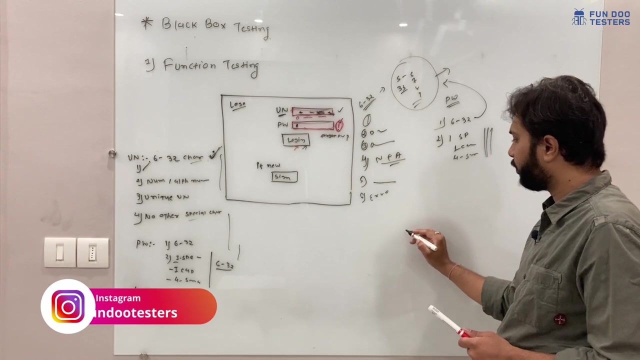 i have to test for one special character, so one special one- capital and four small letters. so i am going to test for the this scenario. so if this two scenario is fulfilled, then what i am going to do, i am going to click on the login button. so 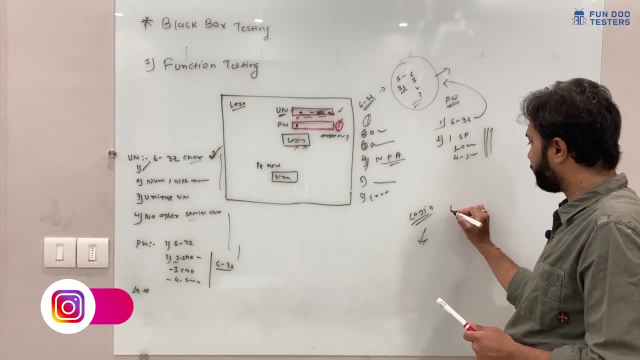 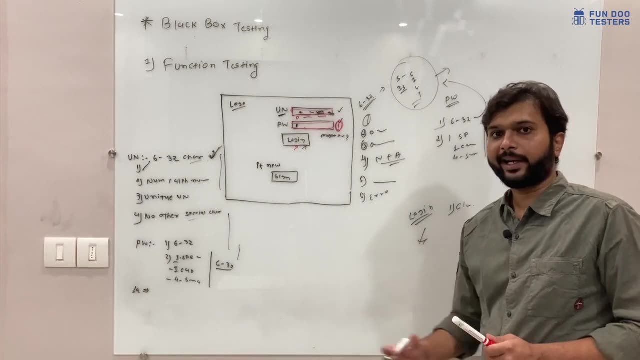 here. after that, login button will come into the picture and i will first time click. after entering the valid data in this group, i will enter, click on the login button. after that i am going to do the negative testing. so the rule of functional testing is we. we are always going to start with. 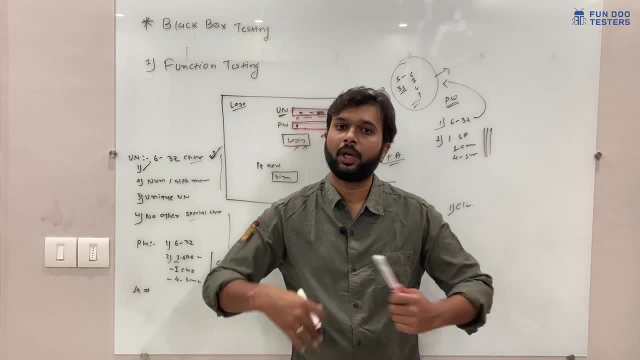 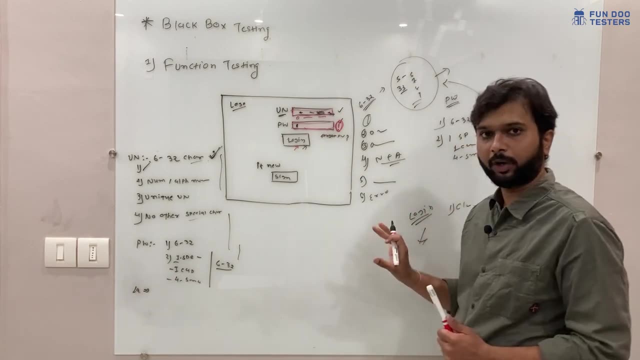 the positive test. once we are able to cover all the positive scenario, then only we are going with the negative data. so here, in this case, i have explained a few positive scenarios. so this scenario we have covered after only we are going with the negative data. so negative with negative data: what 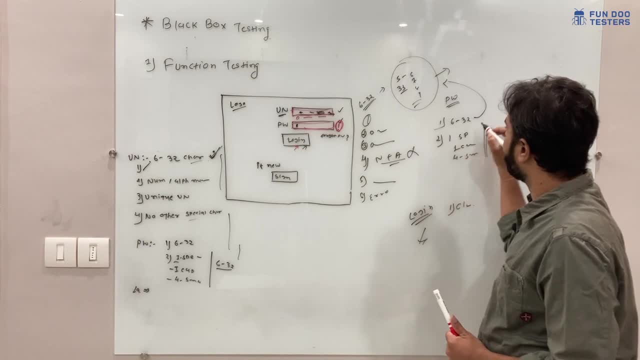 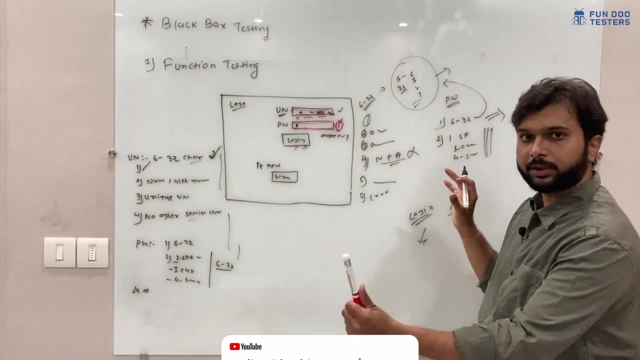 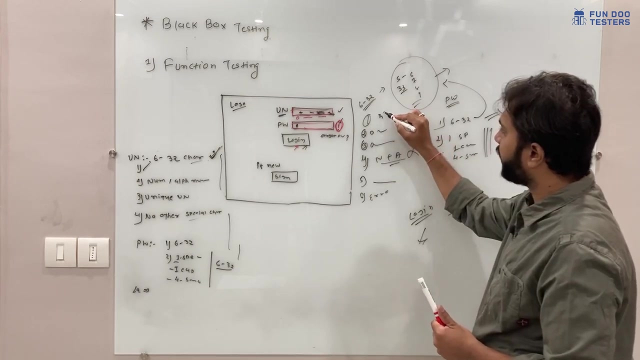 we can do here. we cannot take unique mail id and uh. this combination we are not going to take and we are trying to login, so it will display the error message. so, based on this space, we can write a login test case. uh, we can enter 33 character and then this is the valid data here, valid and invalid, valid, invalid. in all the scenario we are covered very quickly. from then we can start. 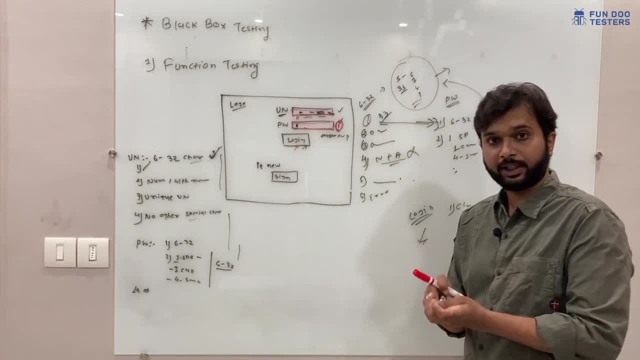 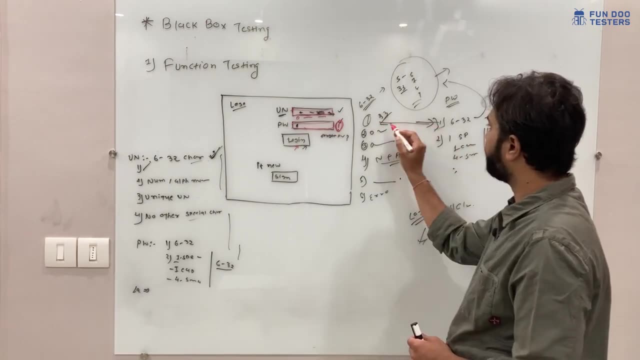 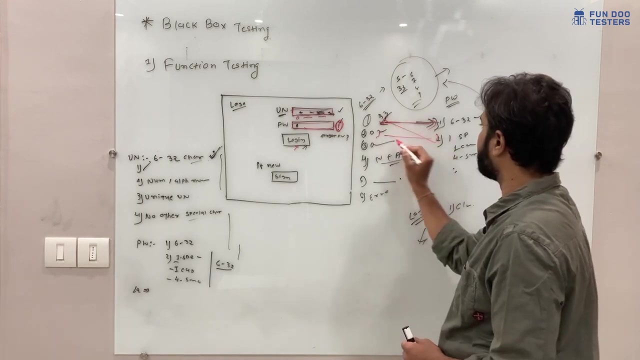 going to test the combinations. so what are the combinations we can test here? so there are multiple combinations we can test as a negative data. so first will be, I will make with the first and first. so one valid, one invalid, one valid, one invalid. so these two, all the scenario later on, first with second, first with third, first with fourth, then second. 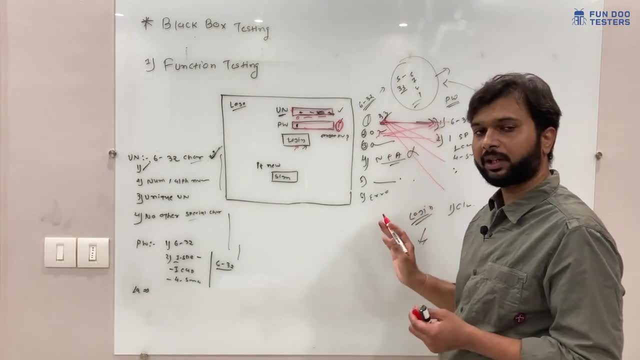 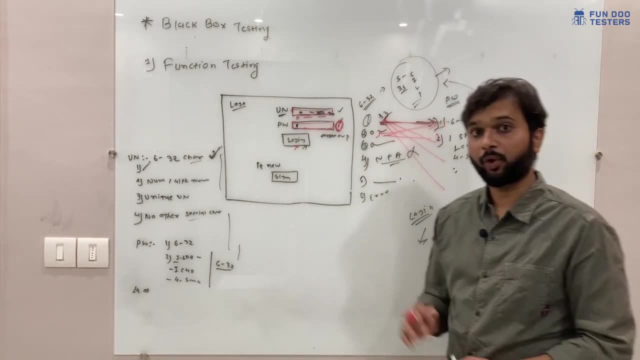 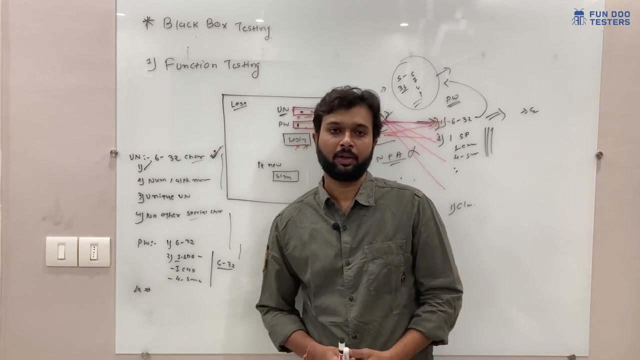 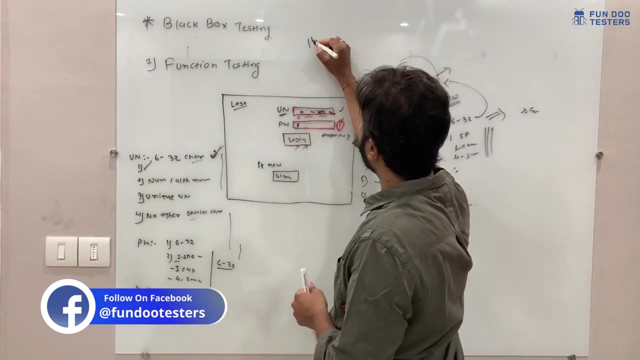 with first. so this kind of permutation and combinations I can make and I can test the login functionality against the requirement. so this is all about the functional testing. now there are few methodology in the functional testing, so there are different ways of doing to do the functional testing. so what are those differences? first is a we can say, first is 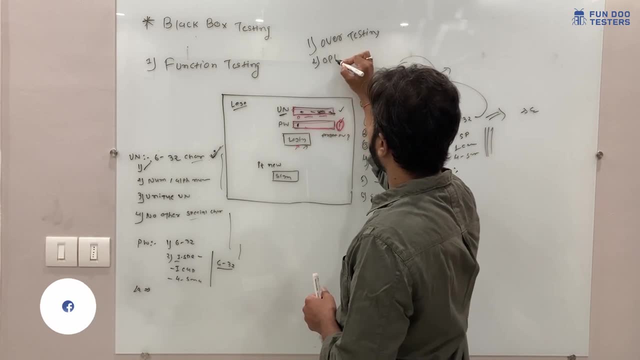 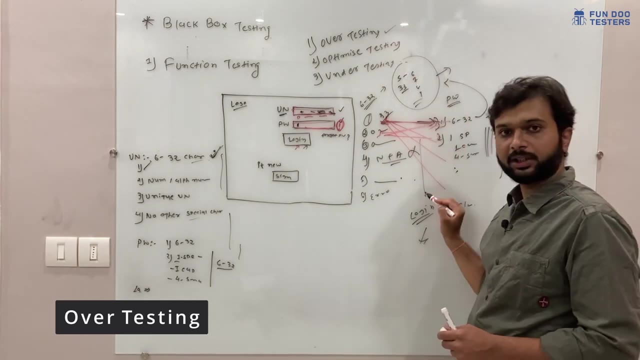 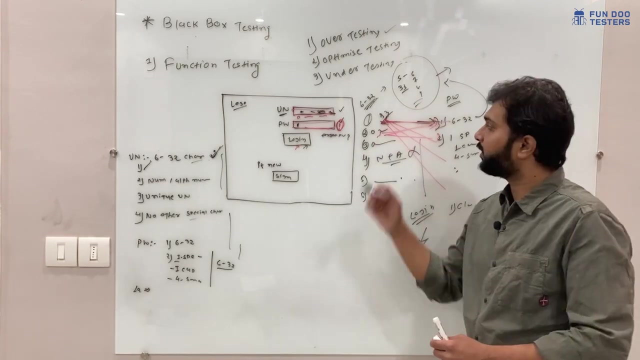 a over testing, second is a optimized testing and third one is a under testing. what does it mean? if over testing means we are testing this scenario in positive manner, so we are testing this data, but what ever, we are going to test multiple times this scenario. 6 to 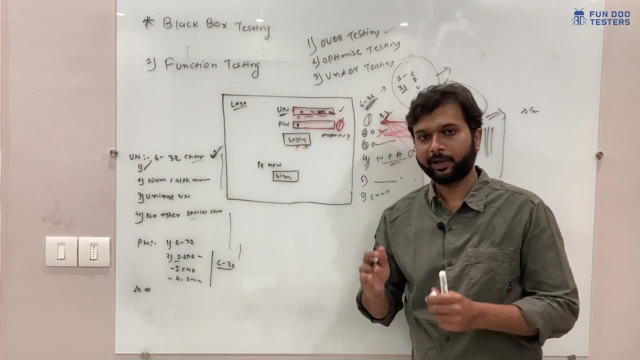 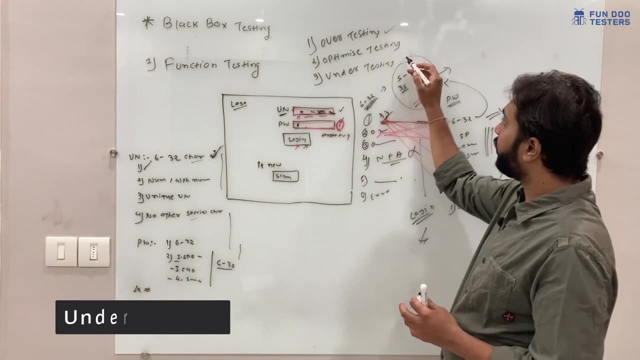 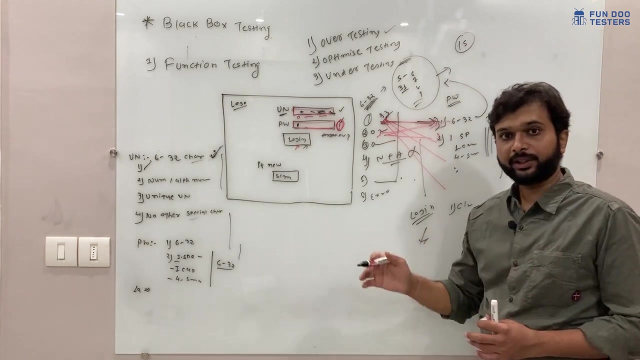 32, 6 to 32 character scenario: we have test once, but we are testing 3, 4 times or 7, 8 times. so that is called over testing later on. under testing means we have to test. for example, we have 15 positive test cases, but instead of testing those 50, we are testing only 10. 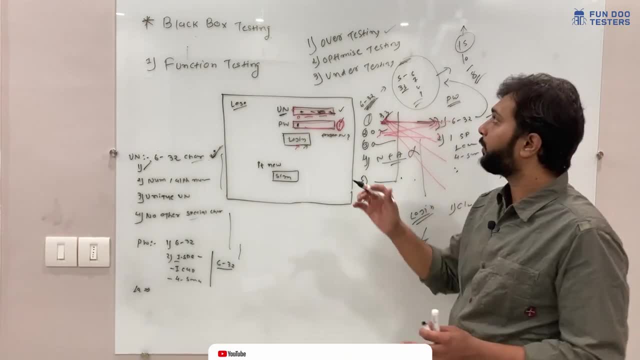 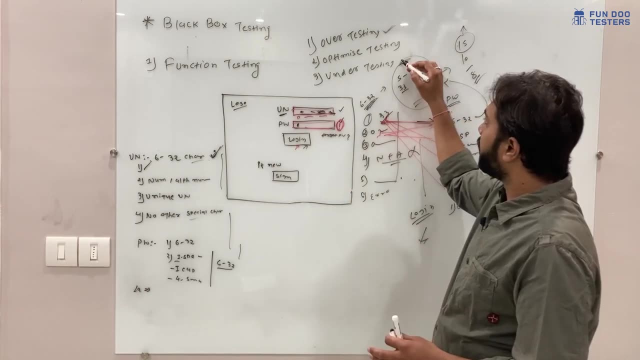 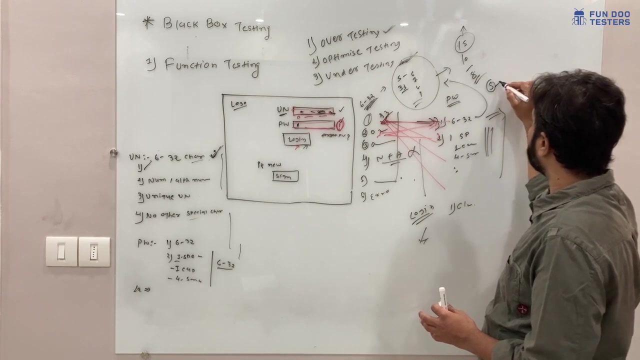 or only 8, so that is called under testing. So what happens? if we are going to do the over testing, then nothing will happen. if we have time we can do the over testing. but what if we are going to do the under testing? so in that case we can miss few box. for example, we have missed here 5 test cases, so there, 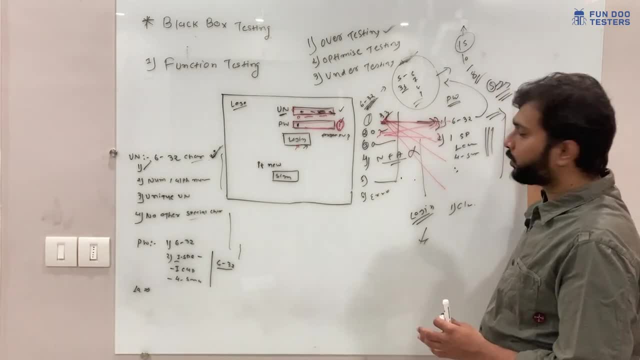 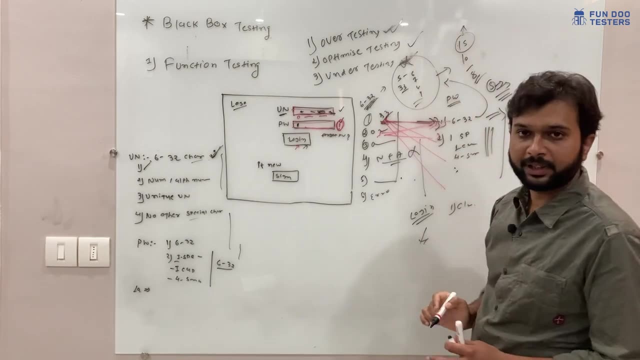 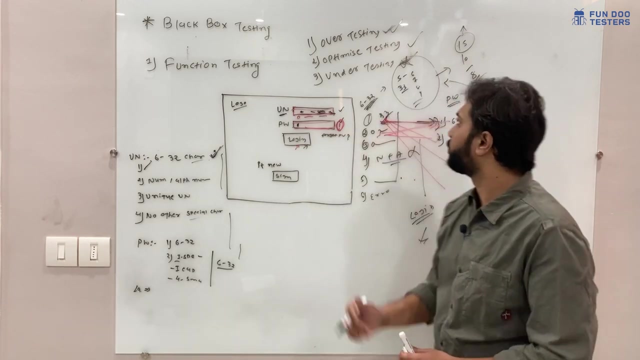 can be a chance. we can find box here. so this box we are going to use under testing is not at all preferable. we can do either over testing or optimized testing. now, what is optimized testing In optimized testing? So whatever the test cases we have, we are going to perform those only so. for example, 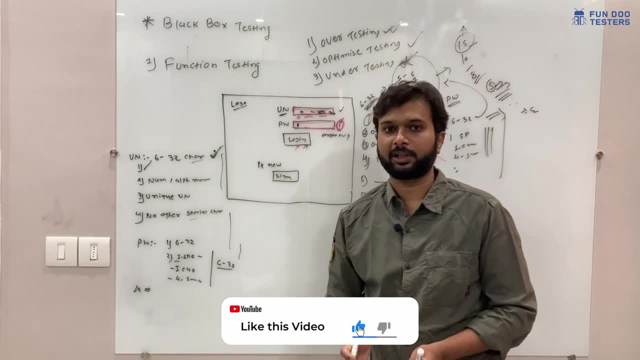 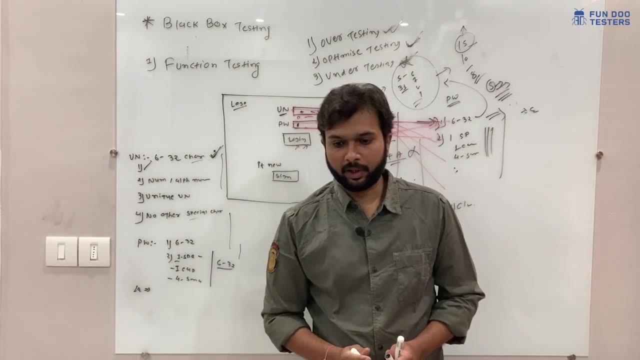 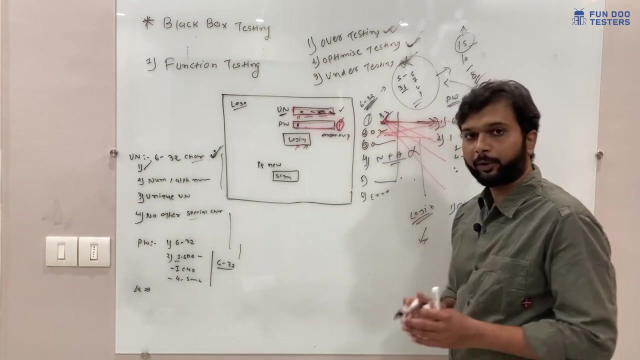 we have 15, then we are going to test only 15 test cases. that is called optimized testing. we can consider this is a perfect way to do the functional testing. Now, another type of testing is positive testing and negative testing. so we have discussed whenever we are going to start a functional testing, we are going to start with the positive 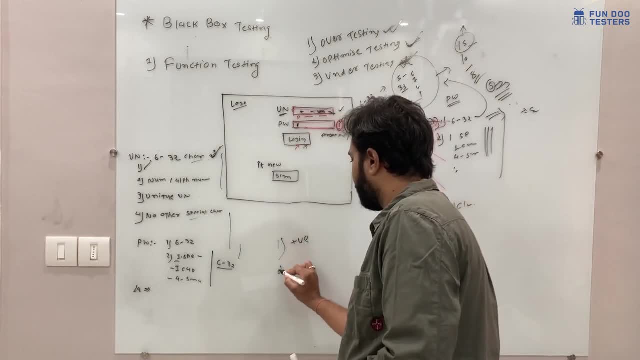 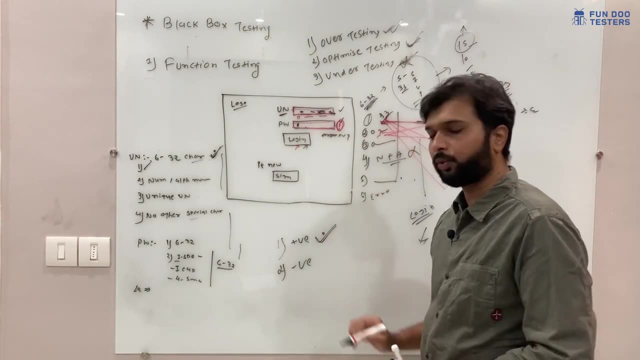 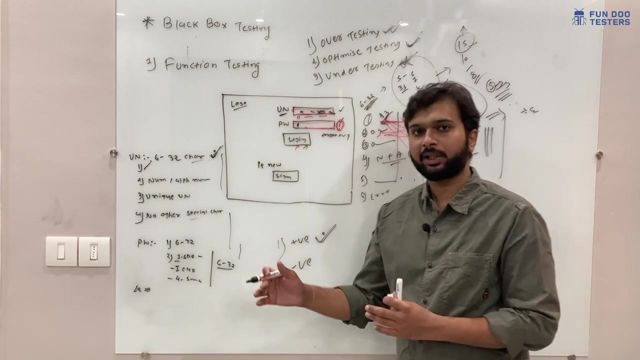 so here we can write positive and negative. So Whenever developer is giving us a new functionality to test, we are going to start. always we are going to start with the positive scenarios. why with positive scenarios? because these scenarios are against the requirement. so we are checking whatever requirement we have. 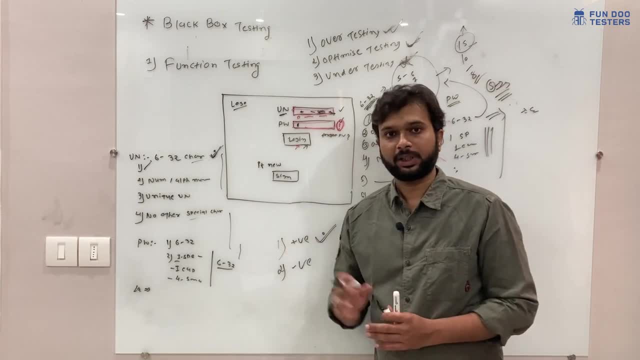 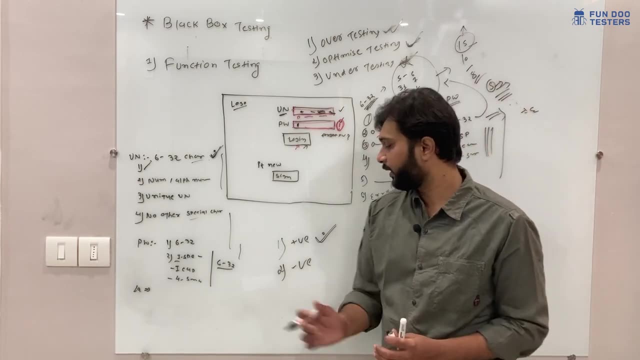 based on the requirement. we are going to check this scenario. we have written those scenario and we are going to test what if we have limited time, if we are running with the out of the time? in that case, if we have missed the positive scenario, also, we are going to test. So If we have missed the positive scenario, so there can be a chance of the bug. but negative scenario, there is no limit of the negative scenario. we can test n number of the scenario and n user is not going to perform those scenario. for example, we have released the application. 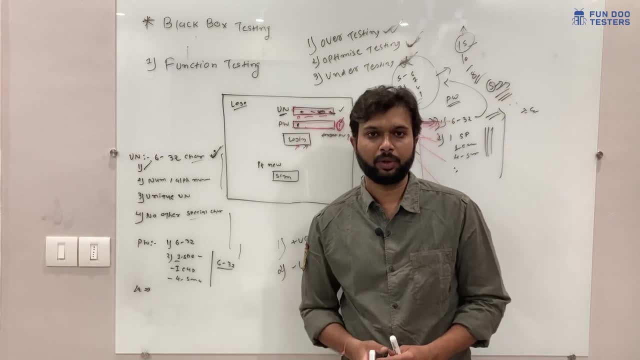 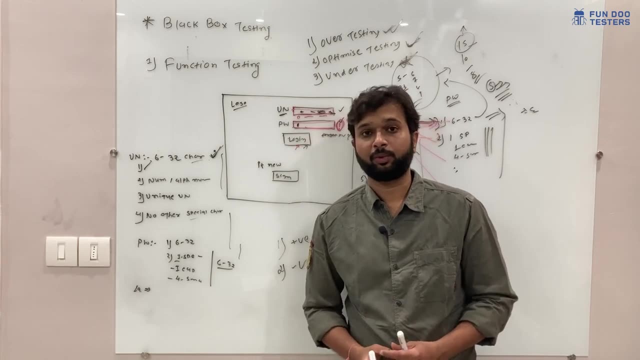 so within one or two days, if we are not going to do the proper negative testing. so user, user also- there are lot of chances that user only can do the positive. just think you are going to use a facebook, so you are a user of the facebook, so you are not going to test. 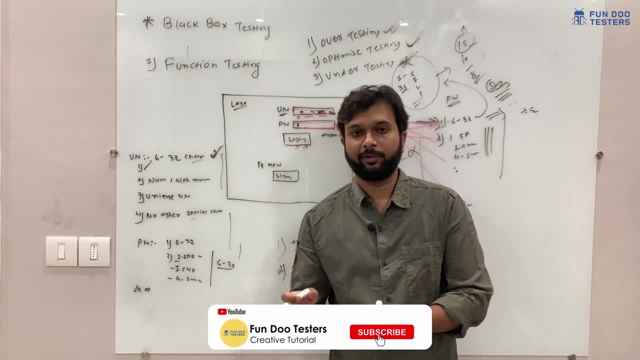 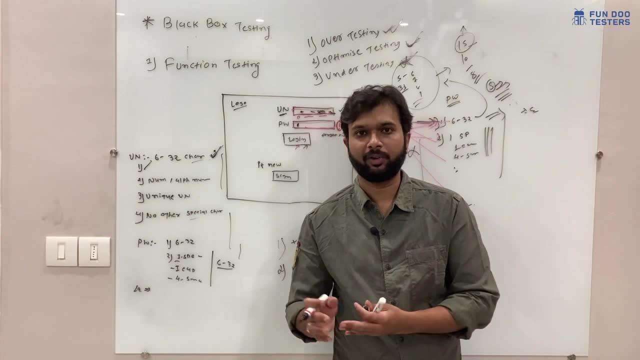 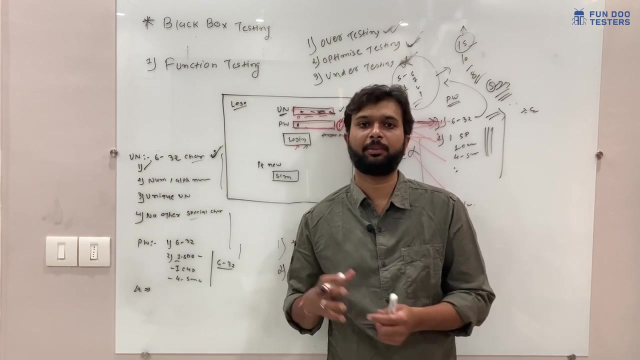 So, So, So yes. so when, if the user says NO, you are not going to enter invalid data or you are not going to test those where but only few user can do, if someone hacker or anyone, they can do or they can try to break the data, or sometimes some people has to post on the linkedin. 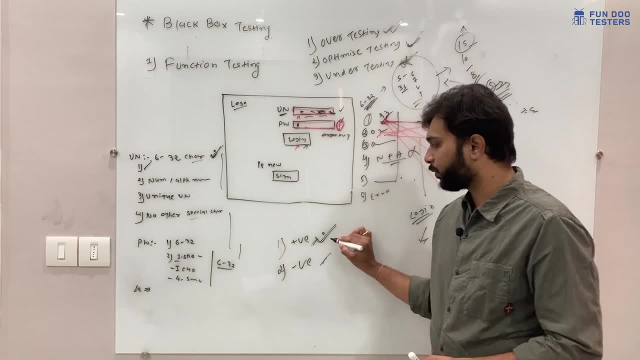 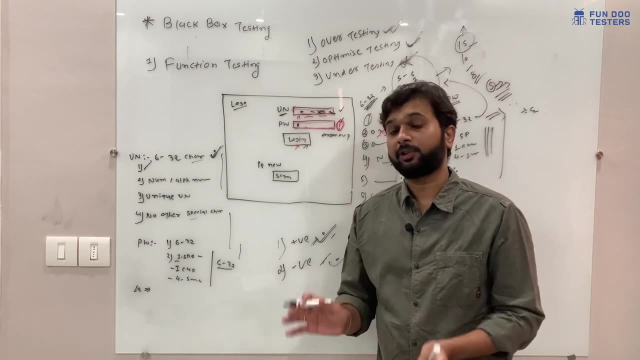 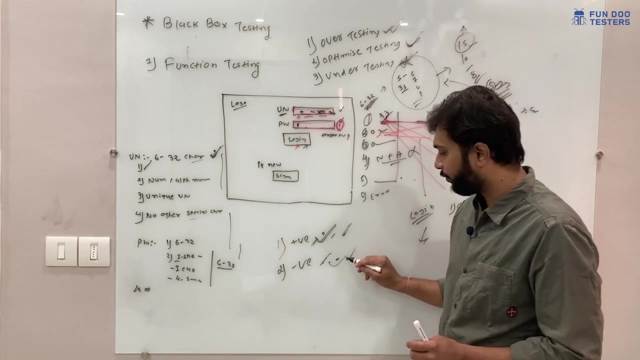 and they are doing that, but initially no one can do so we can do the positive testing one time, we can have more time in that case against the negative test. understand my point. I am not saying, you are not going to do the negative testing first. priority is positive testing. so once positive testing is done, then only we are going.